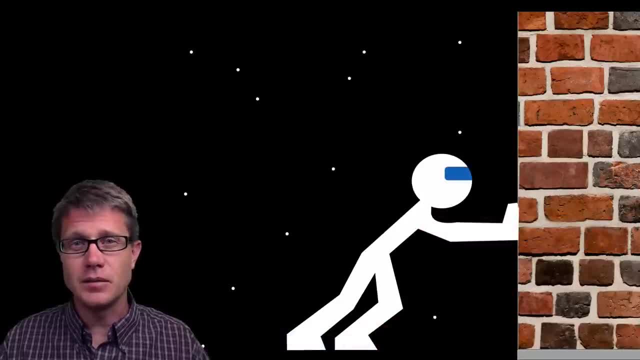 do not accelerate anywhere. Now let's put you in space and do the same scenario And let's make sure that that wall does not move anywhere. So now you apply a force into the wall, It applies an opposite and equal force back on you. And so now, since there is no ground to, 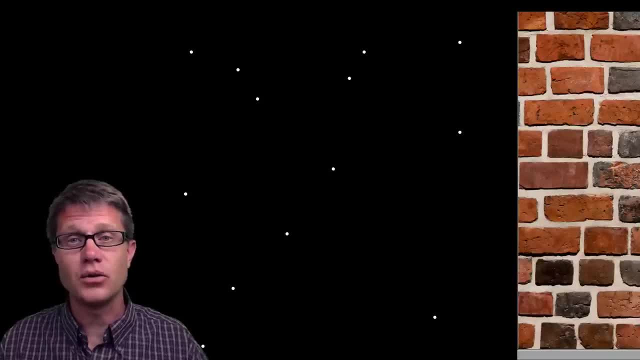 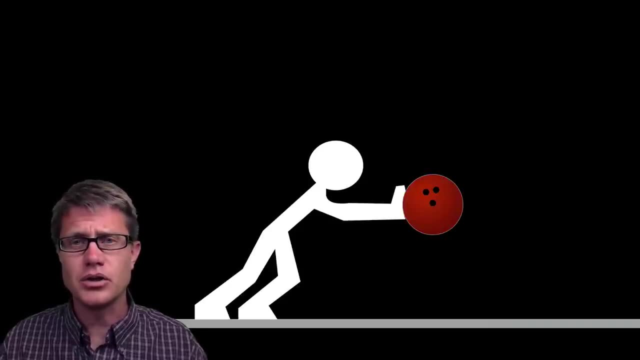 push against. you are simply going to quickly accelerate and then coast away from the wall. Let's look at another scenario. You are pushing a bowling ball And we have kind of frozen at the point at which you are going to push the bowling ball. So you apply a force into. 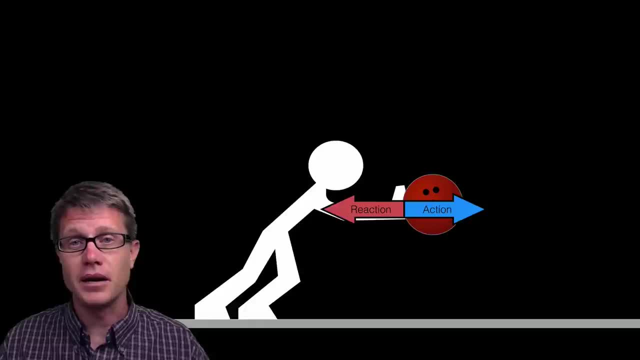 the bowling ball And it is going to apply an opposite and equal force back on you. Now, the ball is going to move, But you are not going to move, And the reason why is you are applying a force against the floor and it is applying a force back on you. 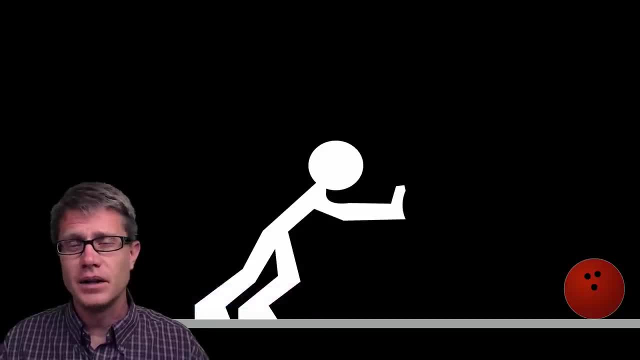 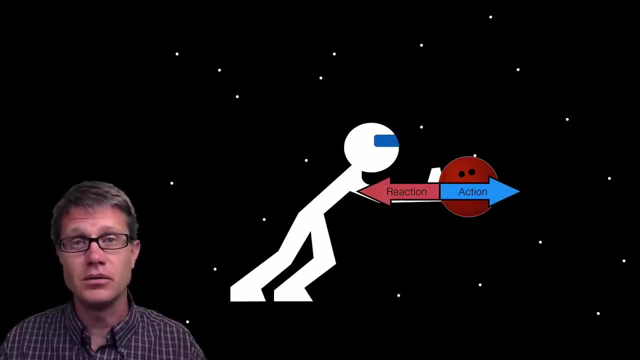 So you do not move, but the ball is going to quickly move away like that. Let's do this scenario again in space. What happens? You apply a force into the bowling ball. It applies an opposite and equal force back on you. What is going to happen now? There is no ground. 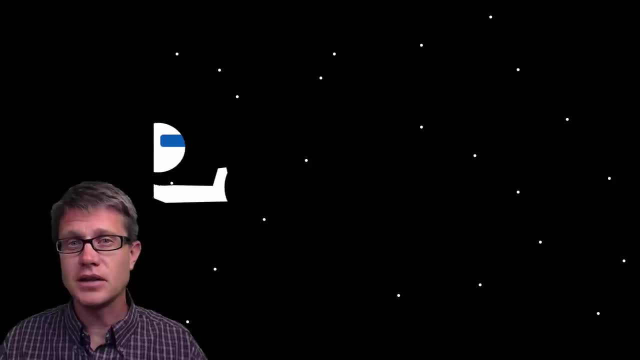 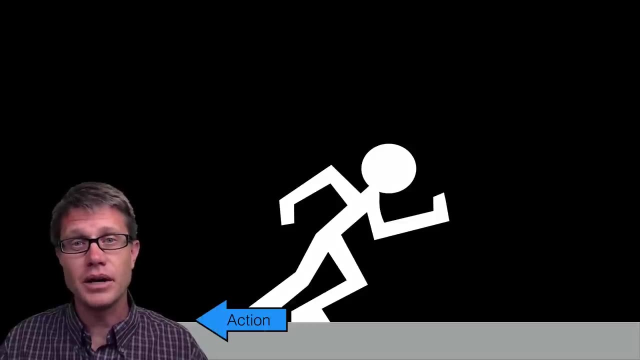 You are both going to accelerate away from each other. Why do not you move as fast as the ball? Because you have a greater mass. Let's look at just walking or running across the floor. You apply a force into the floor and it applies an opposite and equal force. 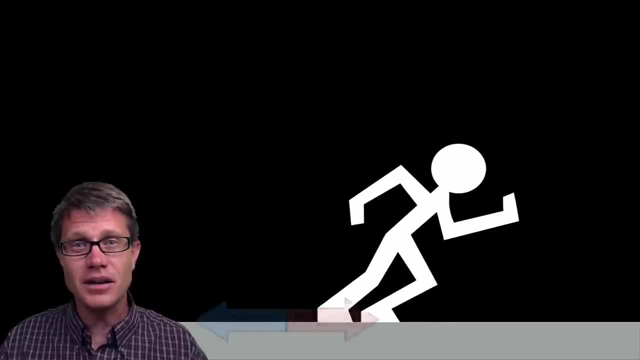 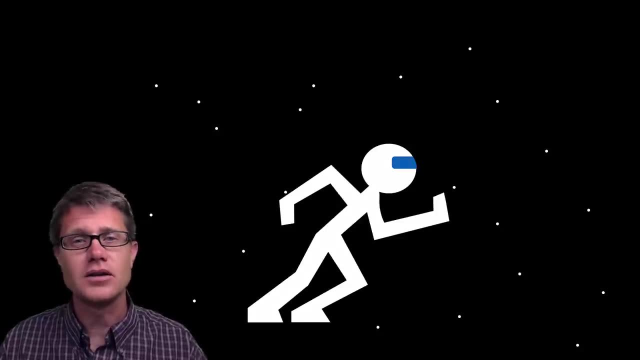 back on you. That does not make sense. But if you think about it in space, what happens? if there is no floor, There is no action. You apply an action, Nothing happens And there is nothing to push against. You are simply stranded there And so these action. 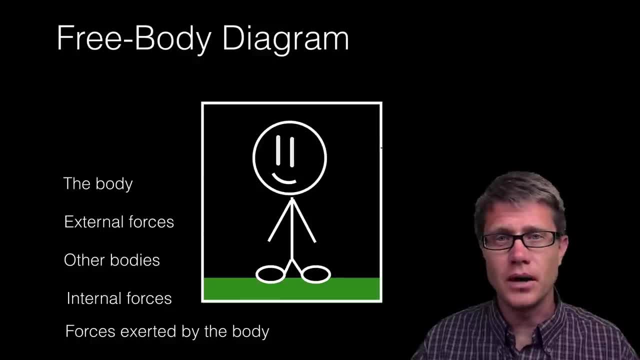 reaction pairs make sense, But it is sometimes hard to figure out what is pushing on what, And so we use a free body diagram to do that. And this is the first time we have used free body diagrams. And so what do you include in a free body diagram? The body. So you are. 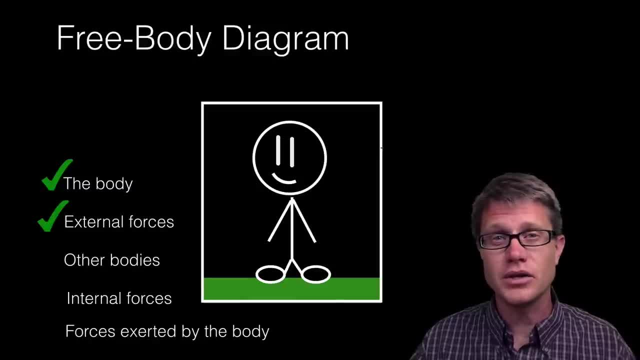 going to include the body And you are going to include any external forces on that body. Now it is more important: what you do not include in a free body diagram. You do not include any other bodies, No internal forces. You, for example, pushing on yourself or parts of 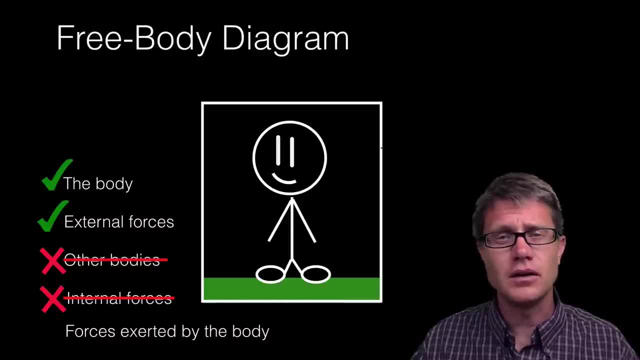 an object, pushing on other parts of the object, And also you do not include any of the forces exerted by that body. That is the one mistake that students tend to make, And so let's do a free body diagram, A few examples, And so if you have a person standing right here on 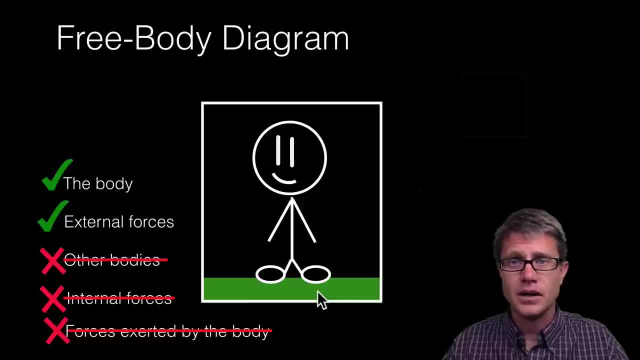 the ground. let's do a free body diagram of their body. So we start. I usually draw a square like this. This represents the body. What are the forces that are acting on that body? Well, gravity is clearly acting on it in the vertical direction. But the person, since they do not accelerate. 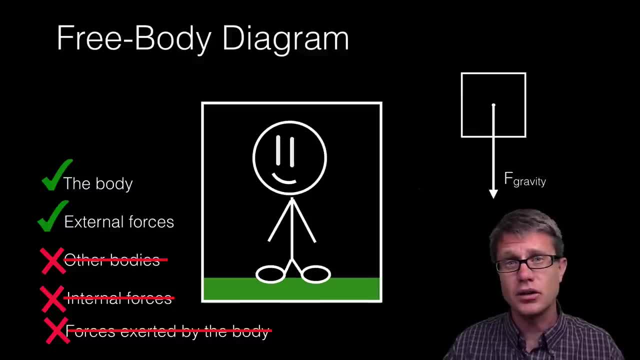 down into the earth. there must be an opposite and equal reaction. That is the ground pushing back on the person, And we call that the normal force, And so those are going to be the two forces in our free body diagram. Let's change it up Now. we are looking at this person pushing. 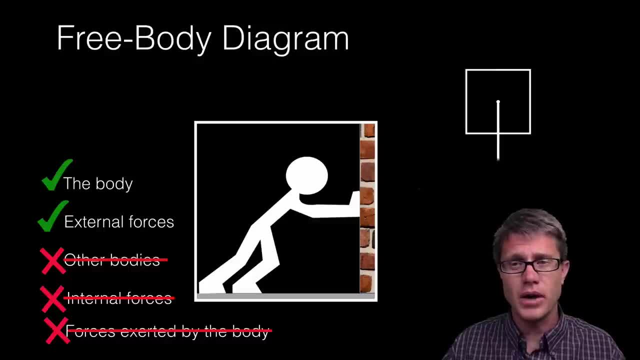 on the wall. So what do we start with? It is always easiest to start with the gravity. So gravity is pushing down. That is an external force. What else do we have? We have that normal force. It is not moving down into the ground. What else do we have? Let's start. 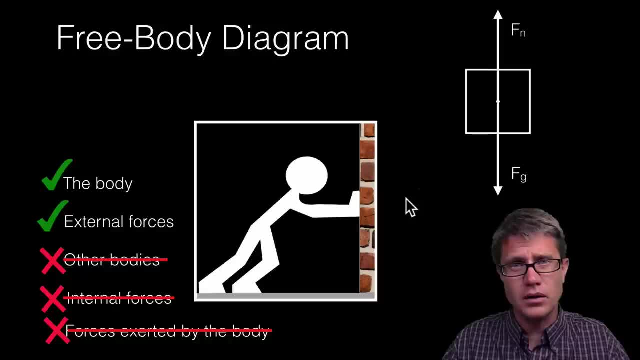 identifying those action reaction pairs. So you are pushing against the wall, But that is a force exerted by the body, So we do not include it. We do include the wall pushing back on you, The force of the wall, If we look at the ground. remember you are applying. 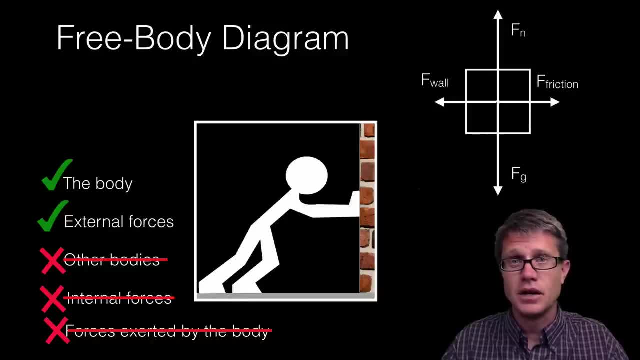 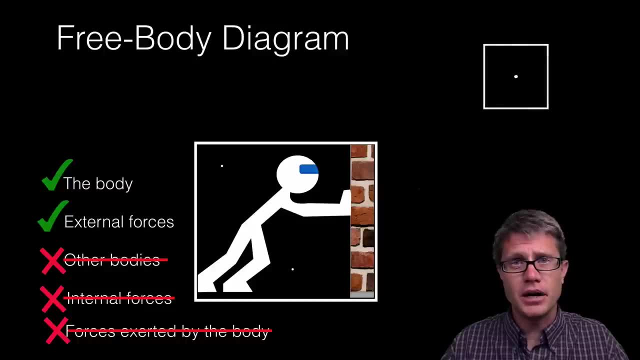 a force in the ground, But there is a frictional force in the opposite direction, And so there is no net force, no net acceleration. If we put that lower force, we are not putting the put this scenario in space. what do we have Now? we have the body again, But there is no. 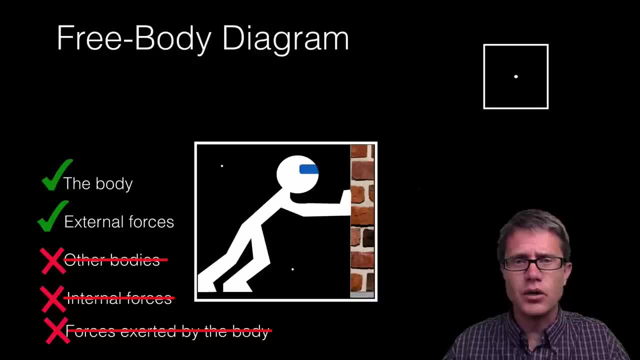 gravity and therefore there is no normal force. We are applying a force into the wall and it is applying a force back on us. So that is going to be your free body diagram. Where is the net force? It is to the left. And so where is the acceleration? It is to the left. 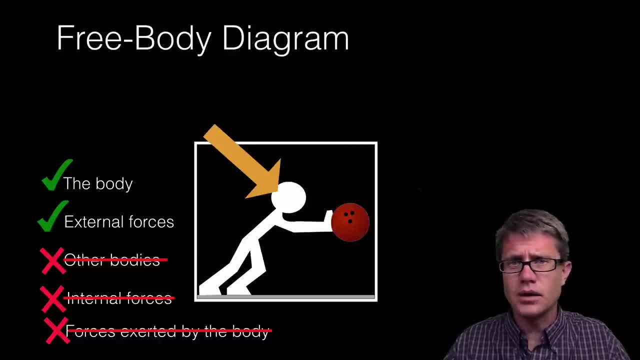 as well. Let's break down these two objects. So we have got the object 1, which is the person, And so we have got gravity and normal force. Those are easy to do right away: You are applying a force to the bowling ball, And so it is going to apply an opposite and equal force. 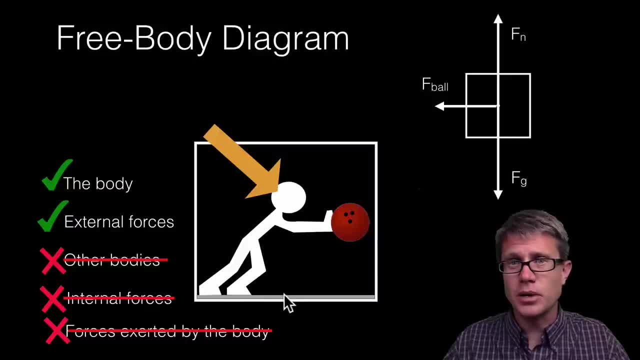 back on you, And then again you are applying a force in the ground And it is applying an opposite force on you, And so we have that frictional force. Now let's shift to the bowling ball itself. So we have again got the object: Is gravity acting on the bowling ball. For 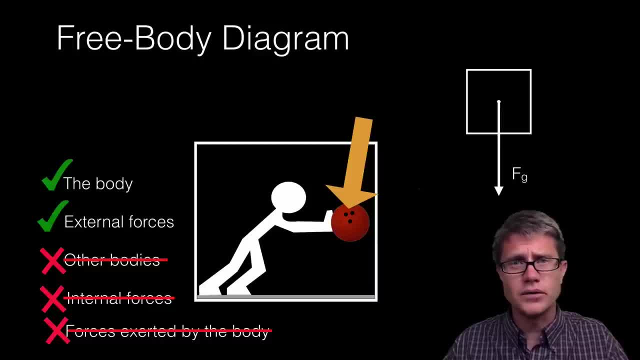 sure, But you are quickly going to let it go. There is no normal force. You have just kind of frozen this picture in time. So there is no normal force. What is the only other external force? It is going to be the person pushing on it, And so where is the force?